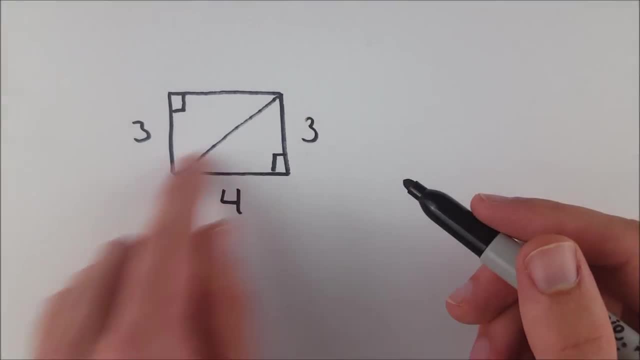 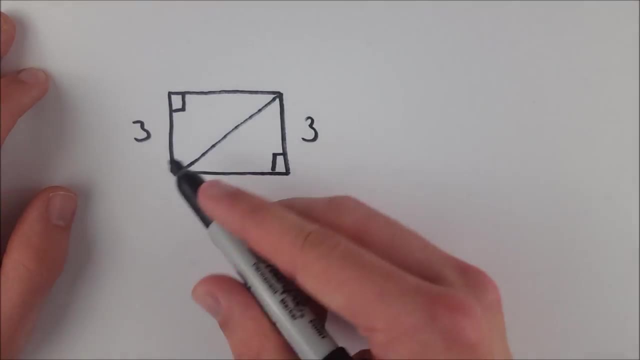 But I'm not going to bother writing that in. And then immediately we've got a right triangle and we know the length of two of the legs. So of course we can just use the Pythagorean theorem to get us the rest of the way and find the length of the hypotenuse. 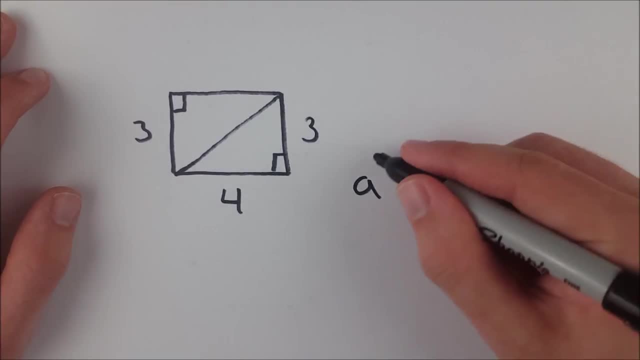 So the Pythagorean theorem tells us that, given a right triangle, the sum of the squares of the measures of the legs, a squared plus b squared sum of the squares of the measure of the legs, is equal to the square of the measure of the legs. 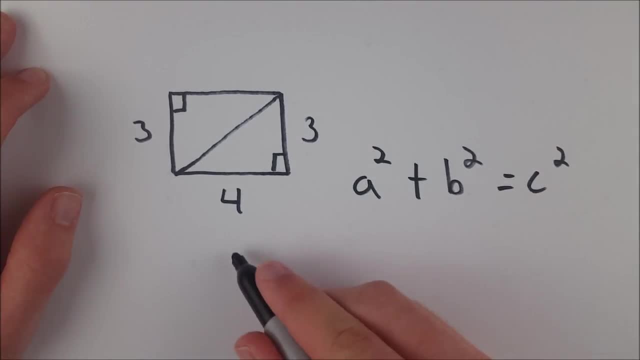 The hypotenuse, which is c squared. So we get 4 squared the square of this leg, plus 3 squared, the square of this leg is equal to c squared. I could have made this d squared, because this is our diagonal, but we'll just call it c because that's what we're going with at the moment. 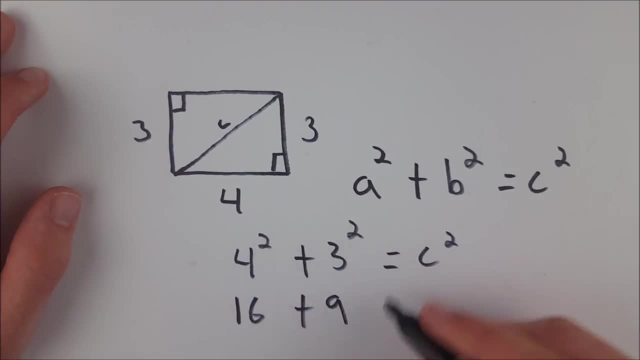 So this leaves us with 16 plus 9 equals c squared, So 25 equals c squared. Of course, you take the square root of both, Both sides, and you are left with c. Square root of 25 is 5, so c is equal to 5.. 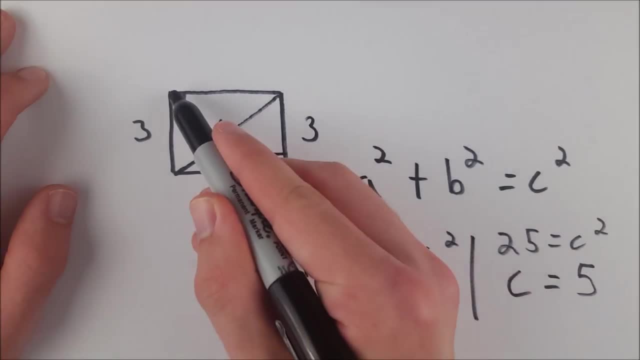 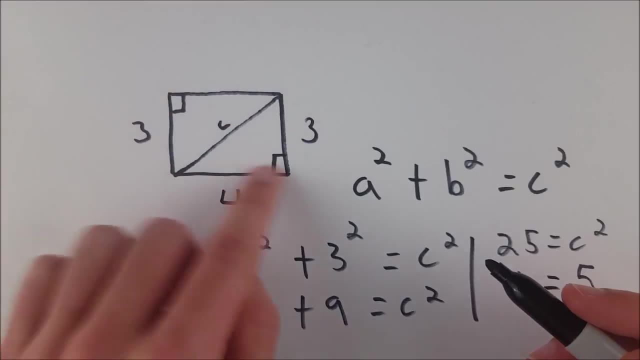 So we know that the length of our diagonal is 5, and, additionally, the length of the diagonal running this way is also equal to 5.. So all you have to do, if you know the length, the dimensions of the rectangle, the length, the width, then you can use those to find the length of the diagonal. 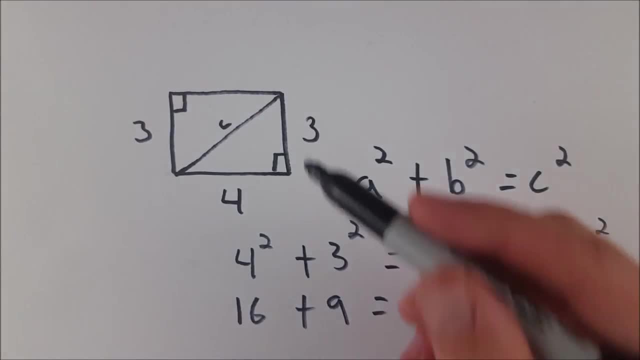 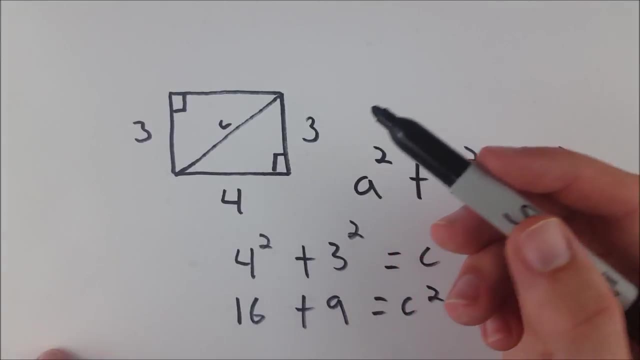 By using the Pythagorean theorem, you just have to take the square root of the sum of the squares, Of the side lengths, the non-congruent side lengths, I should say, although they might be congruent if you're working with a square which, of course, is a subset of rectangles. 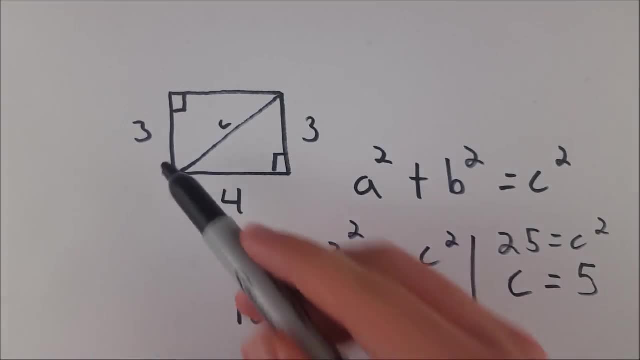 But in any case, this is how you do it. It's just a quick little Pythagorean theorem and then you find the length of the diagonal. So I hope this video helped you understand how to find the length of a diagonal of a rectangle. 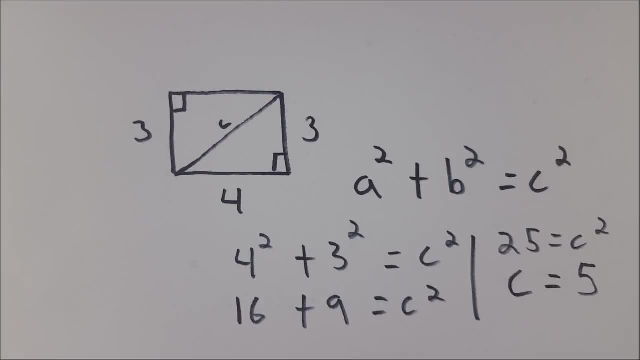 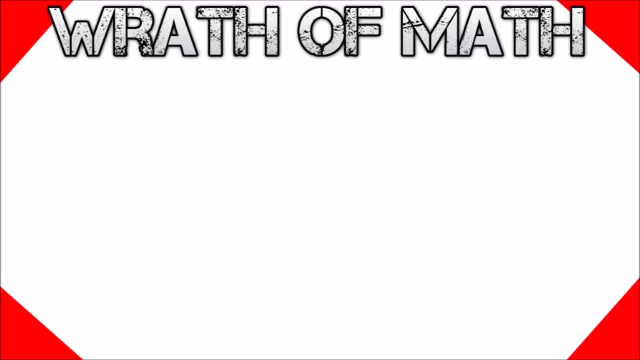 Let me know in the comments if you have any questions or need anything clarified. I'll see you next time and be sure to subscribe for the swankiest math videos on the internet All the way up here. dear, Won't you please come to me?